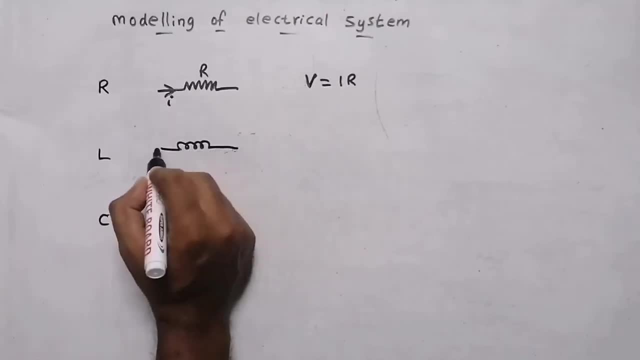 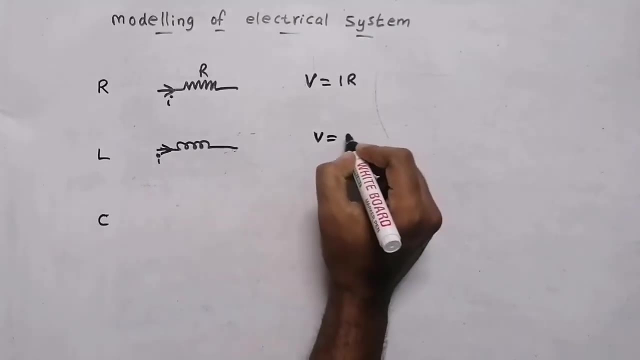 across resistor. Now suppose, think that there is an inductor and through this inductor a current is flowing. Then what will be the voltage across this inductor? How to find the voltage across this inductor? According to Faraday's law of electromagnetic induction, we know voltage across. 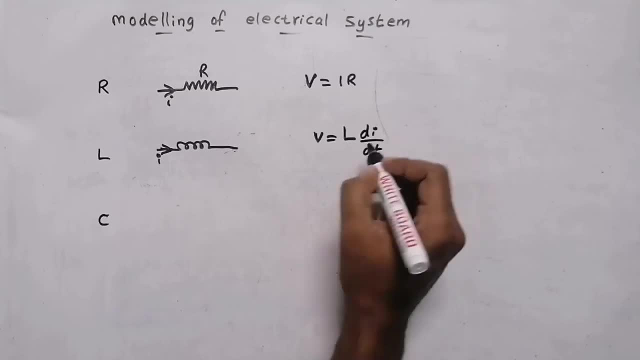 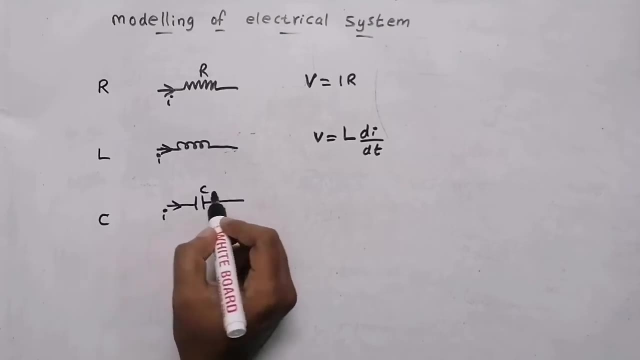 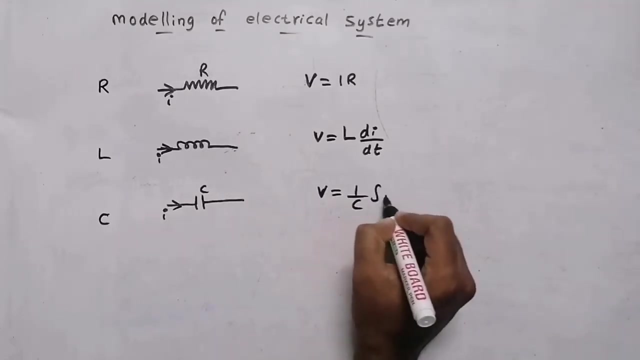 inductor will be change in current by change in time: L, di by dt. Okay, now there is a capacitor and a current is flowing through this capacitor- C, Okay. so what will be the voltage across this capacitor? How to find the voltage across this capacitor? Voltage across the capacitor will be 1 by C, integral I, dt If you. 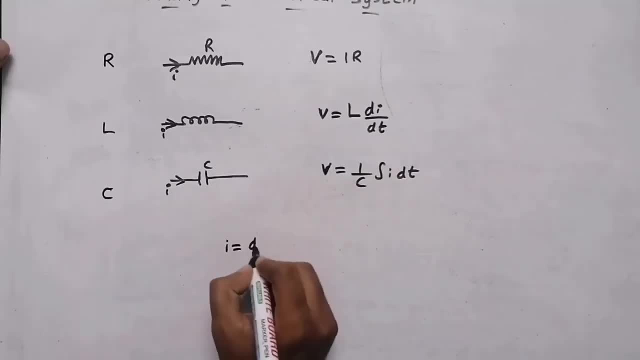 don't know how to find this equation, I will show you. We know current I equal to dq by dt, Change in charge, by change in time. Okay, from this we will get dq equal to idt. So we know current I is 1 by C, integral I dt. Okay, now we need to find q. What we need to do? we need to integrate both. 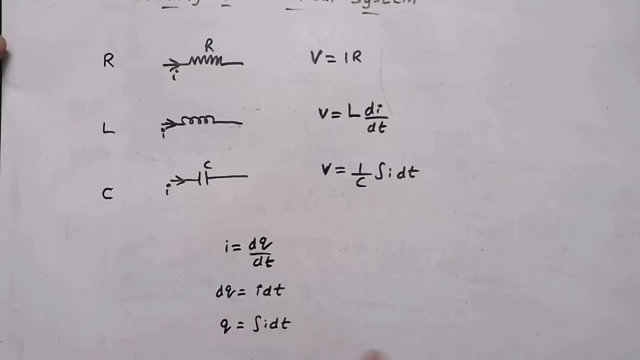 sides. So we will get q equal to integral idt. Okay, and we know capacitance, C equal to q divided by V. that is charged by charge by voltage. Okay, now from this we need to find voltage, So you'll write V equal to q divided by C. and we already found q equal to integral idt, So you'll write: 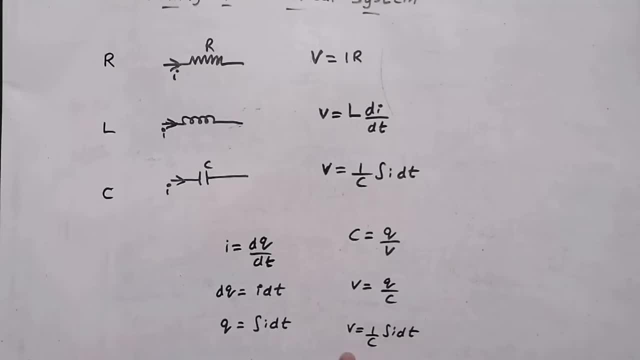 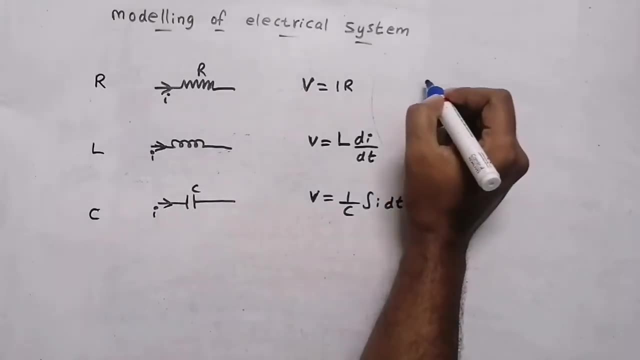 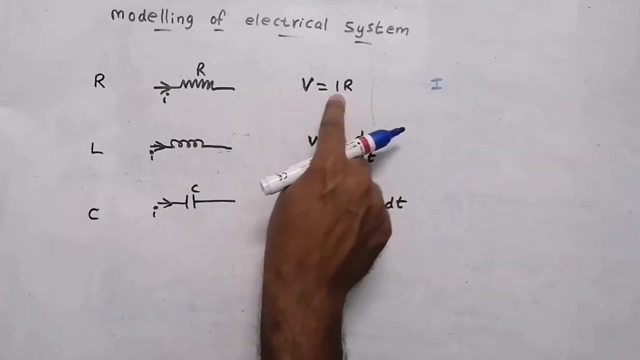 V equal to 1 by C integral idt. Thus you will get the voltage across capacitor. So we found voltage across each element. Now we need to find the current across this resistor. We have found all the voltages, Now we need to find current. Okay, so for finding current, we know V equal to Ir, So I 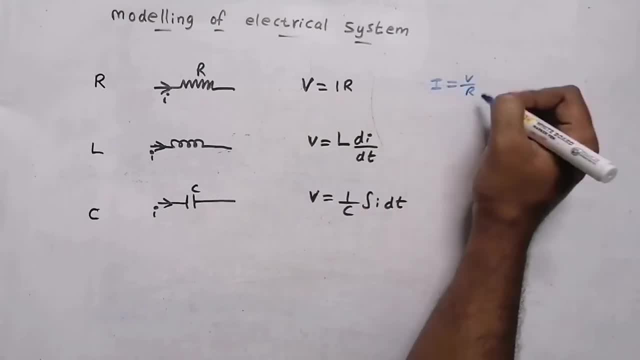 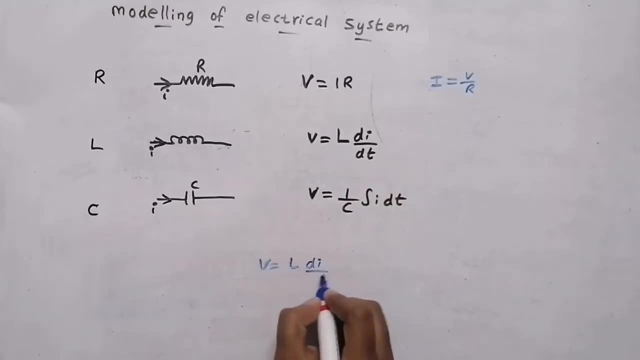 will be equal to V divided by R. So current across resistor will be V divided by R. Now we need to find current across this inductor from this equation. How to find that? I will show you. We know V equal to L di by dt. From this we can write V dt equal to L di. Then we can move this L to. 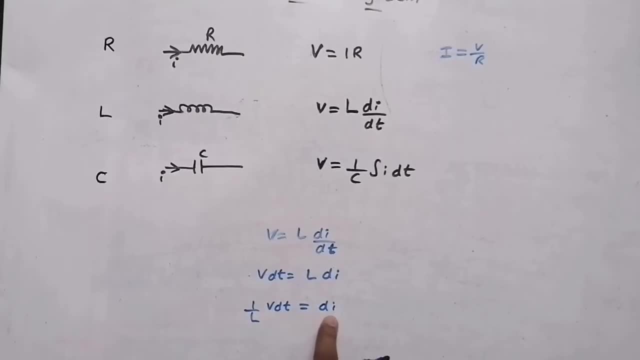 equal to di. Now, here it is di, but we need i. i means current. So what we will do, We will integrate both side, Then this d will go, Then we will get i, and here 1 by L is constant, So I will. 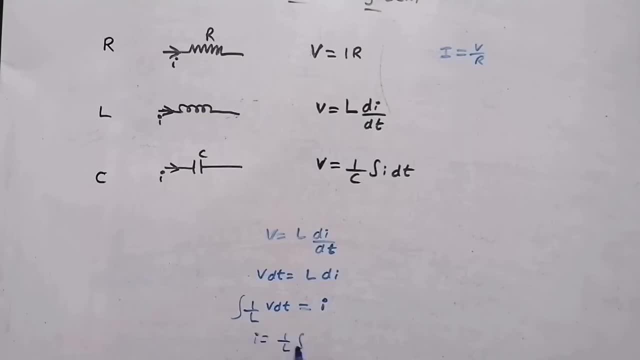 take it outside, So you will get i equal to 1 by L integral V dt. So from this equation we will get i equal to 1 by L integral V dt. Same for capacitance. We need to get the current i, So we 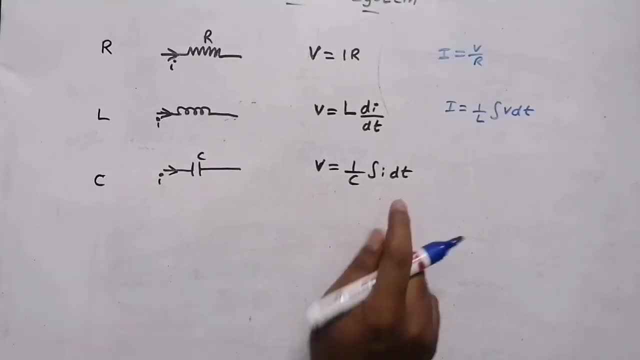 need to differentiate both side. We have this equation. From this we need to find i. So I will first multiply now, So Cv equal to integral i dt. Now, for removing this integration, what we will do, We will differentiate both side. Now C is a constant, So I will take C outside Then. 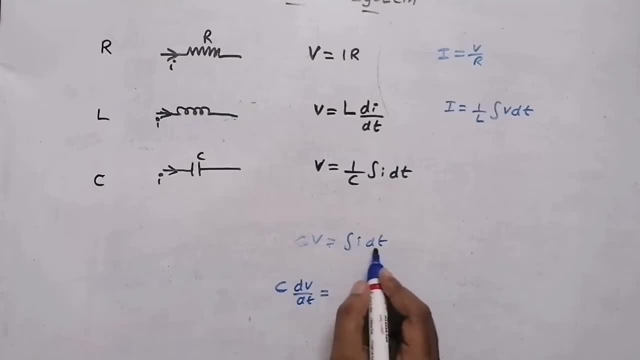 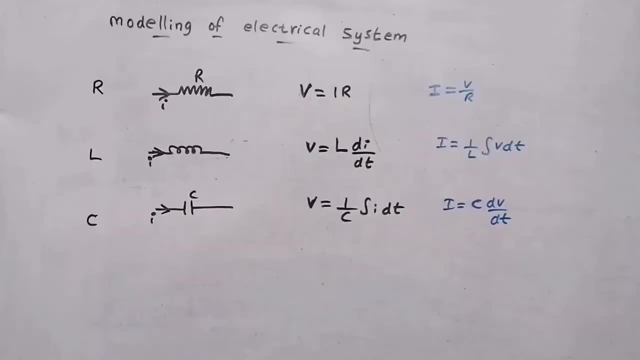 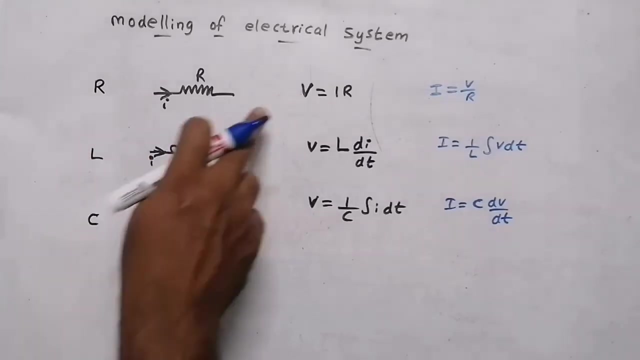 differentiating dv by dt equal to, Then this side differentiating we will get i. So from this we will get i equal to C dv by dt. So this is the basic thing we need to know for modeling an electrical system. There are three elements: resistor, inductor and capacitor. We need to 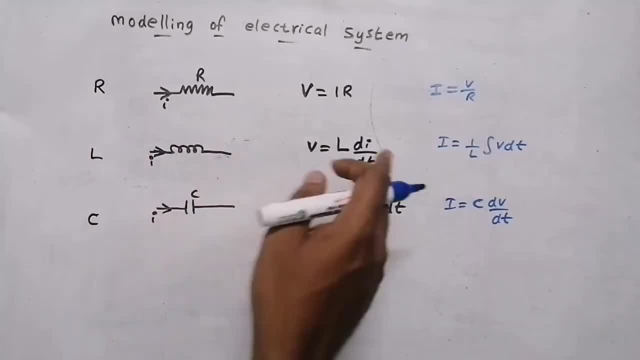 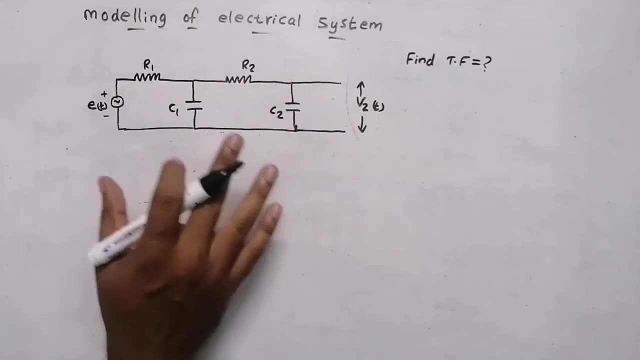 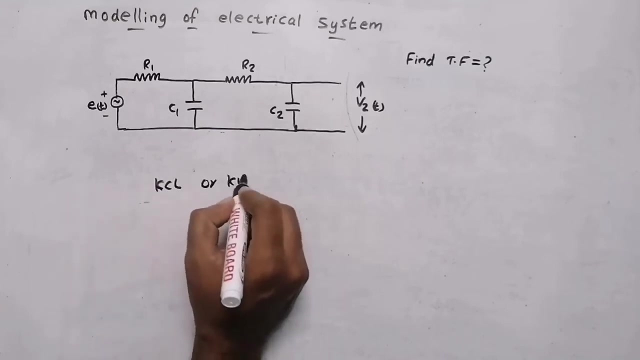 find the voltage across each element, We need to know the equations. Then we need to know the equation for finding current across each element. So in this question we need to find the transfer function of this electrical system. So how to do that? Okay, So first of all we need to use either KCL or KVL. Okay, In this system, either we can do. 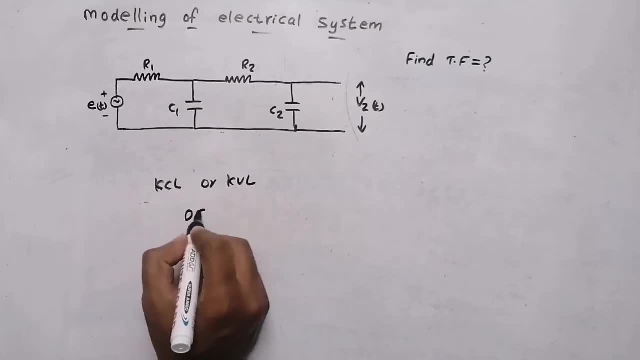 Kirchhoff current law, or we can do Kirchhoff voltage law. Then we will get a differential equation. But solving differential equation is not easy. So what we will do, We will convert algebraic equation is easy. So algebraic equation, How we will convert differential equation to. 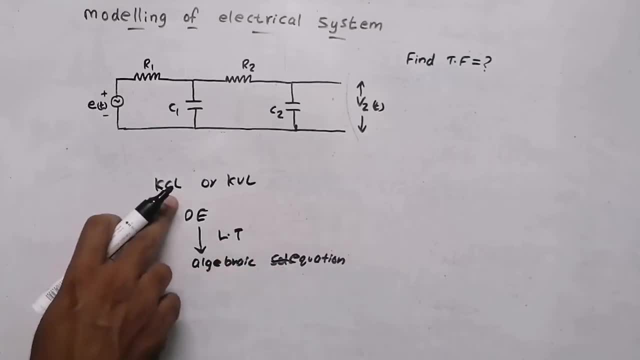 algebraic equation Using Laplace transform. So first of all we will do either KCL or KVL, Then we will get a differential equation. Then we will convert this differential equation into algebraic equation using Laplace transform. Now we got the algebraic equation, Then we will write. 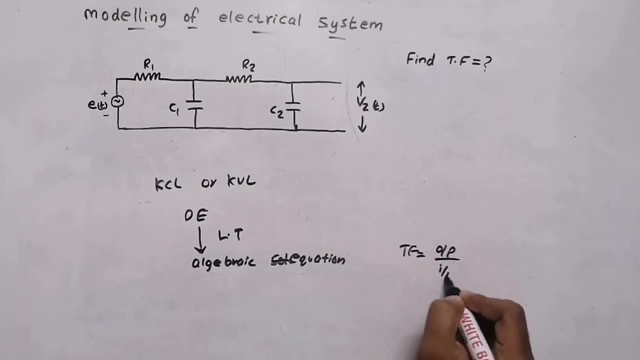 transfer function by using ratio of output by input. Okay, In this case the ratio of output, Output is here, it is voltage. Okay, So output is a voltage b2 and input is the voltage source. Here that is e, And now it is in time domain, That is, in bracket, it is t, That means time. 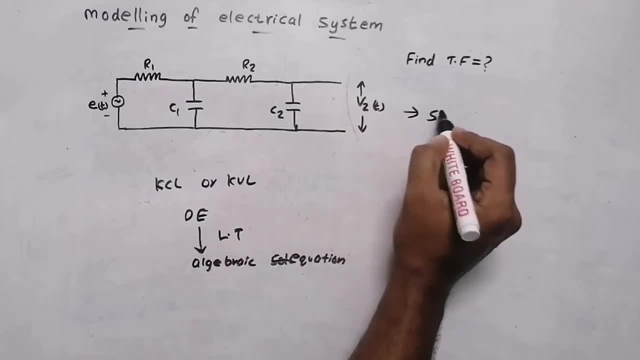 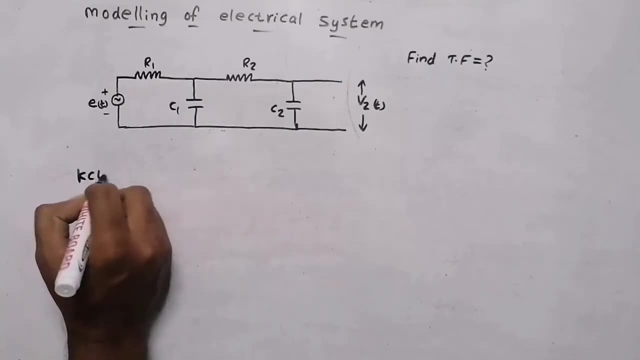 domain. When we do Laplace transform time domain will be converted into s domain. Okay, So first of all we need to write either KCL or KVL. I am going to use Kirchhoff current law, That is, sum of current entering a junction will be equal to sum of current leaving the junction. So I am going 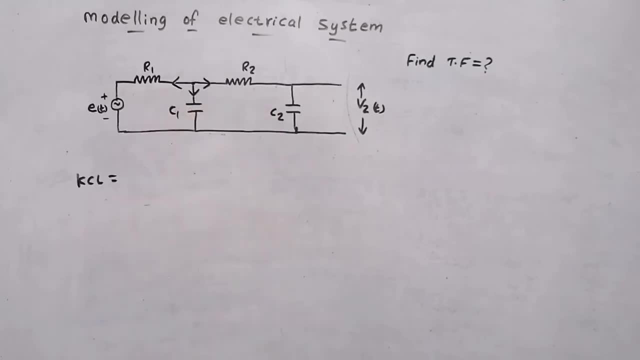 to denote the current as leaving the junction. This is my junction and the voltage at this junction I am going to name it as b1.. Okay, Now, at this node also, I am going to assume that current is flowing away from this junction and I am going to name the voltage at this. 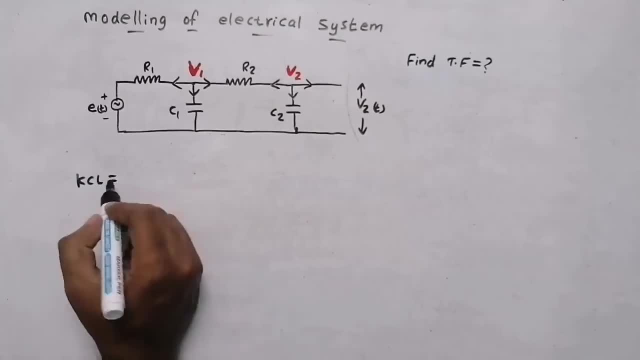 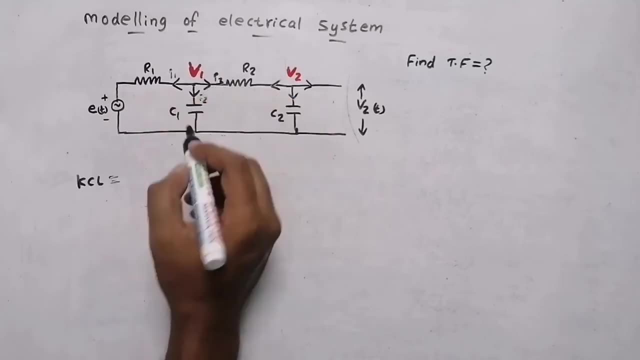 junction as v2.. Okay, Now I am going to apply KCL in the first node. So this current it is I1.. Here it is I2 and here it is I3.. So, according to KCL, sum of current I1 plus I2. 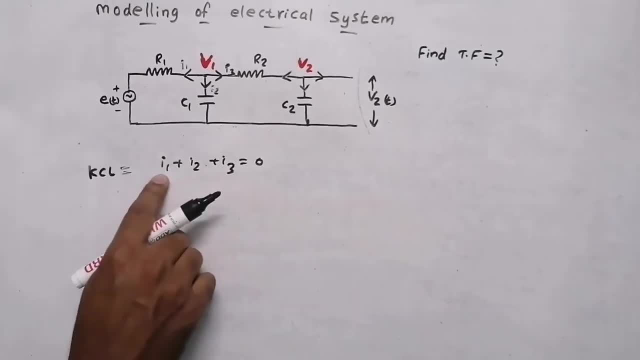 plus I3 will be equal to 0.. Okay, So first of all we can find I1.. I1 is the current flowing through resistor, So we already found current flowing through resistor. it is V by R, voltage by resistance, So we have voltage here, V1 and we have a voltage source E. So we will write V1 minus E of T. 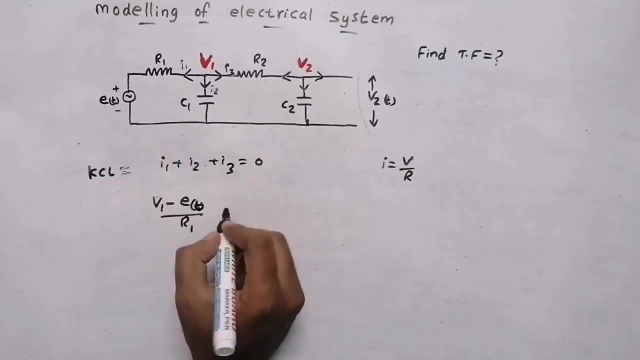 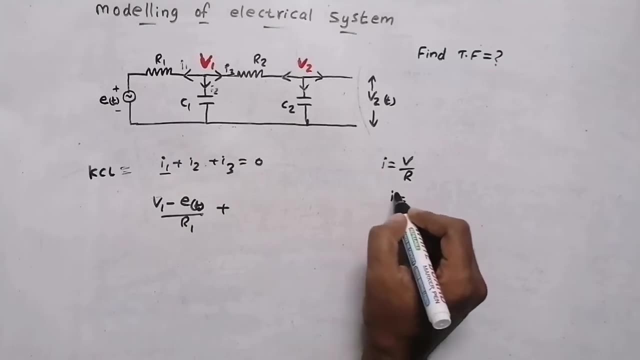 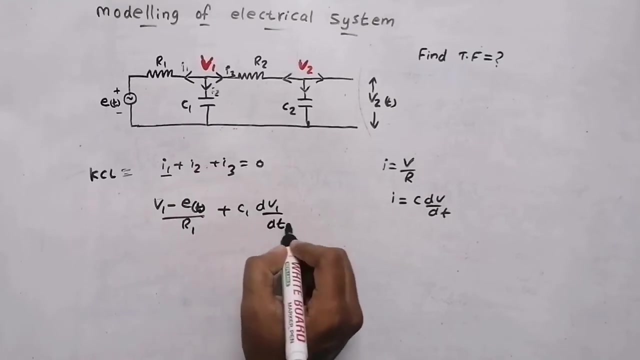 in time domain. Okay, Divided by R1.. So that is our I1. Now we wrote I1.. Now we need to find I2.. I2 is the current flowing through this capacitor. So we found current across capacitor. it is C, dV by dt, So in this case it is C1.. So C1, dV1 by dt plus I3.. I3 is the. 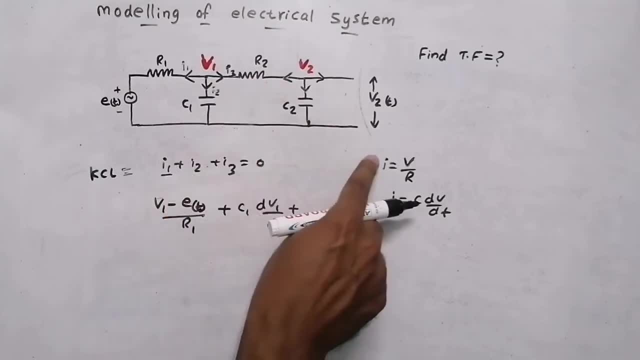 current flowing through this resistor R2.. And we know current across resistor it is V divided by R2.. Can you see, now we have such total force, I this time over power, I2 over R2.. Hey, I have total in it. now there is a slight wear on participate in the flow through this capacitor. 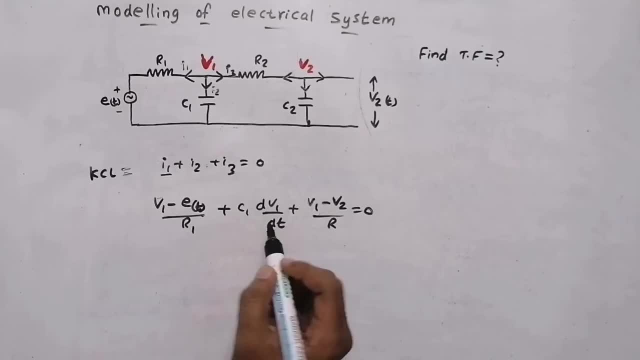 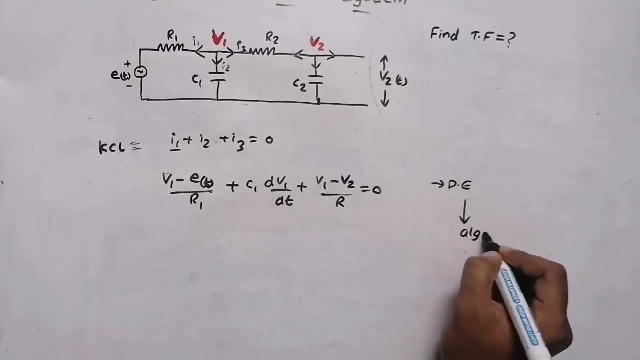 And, as you can see, I should get the output as V2.. Here, baby, V2 and c is equal to Bt. we got Darth aqui, but here we have V1 and V2.. So see how well the Brillouin line can work as sitting here, Cont Lakes, way upwards from. 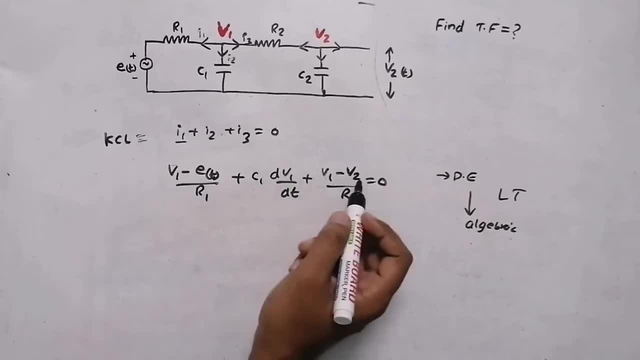 the time level to, as we have cardee V2, now I had changed V2 into 1. So in the future will be same so far. so so in the future we will of course plug KCLเช to. hereit is our voltage through resistor. So we will look at V2 and V3 also, but here we have V1 and V2.. 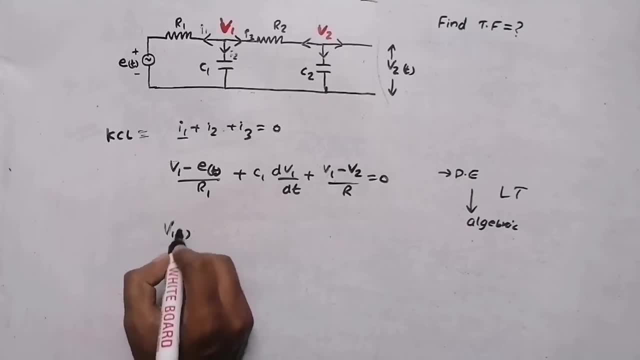 So we will write V1 minus V2 divided by R. wwe will write V1 minus V 2 divided by R. that is equal will be converted into capital v1 of s. so here it was in time domain. we will convert that into s domain in laplace transform minus small letter. e of t will be converted into capital e of s. 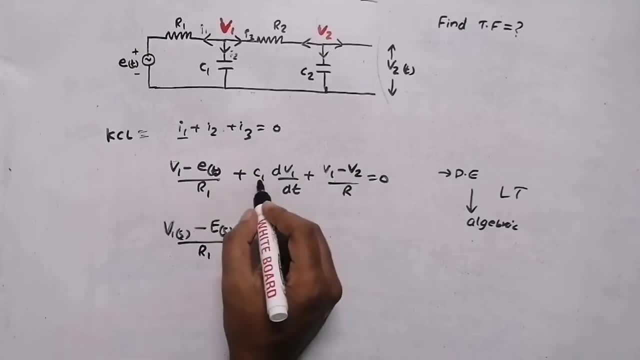 then r1. it is resistor. that is a constant. we will write like that itself, then c1. c1 is also constant. we will write like that now: dv by dt. in laplace transform it will be s. if it is d square by dt, then it will be s square. if it is d cube by dt, then it will be s cube. here it is dv by dt. so 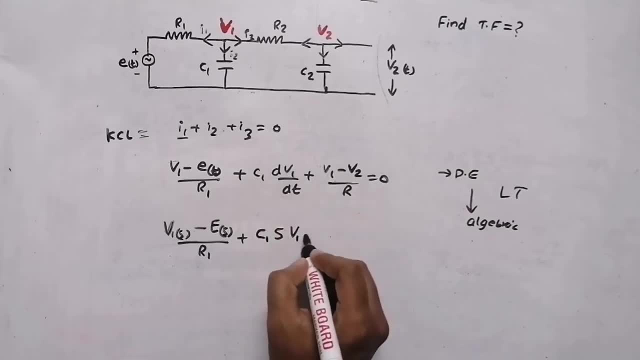 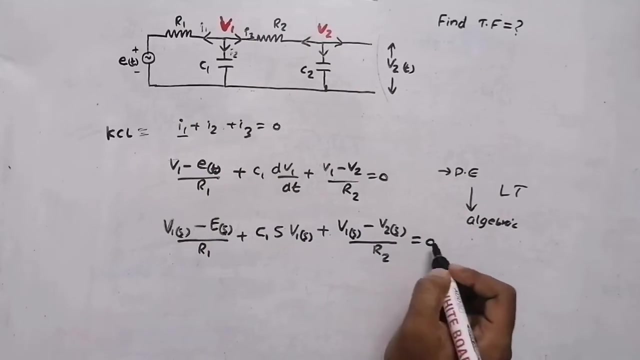 we will write s now. small letter v1. we will write into capital letter v1 of s in s domain plus v1. small letter v1 will write into capital letter v1 of s minus small letter v2 will write capital v2 of s divided by r2. this is our r2. okay, resistance r2 that is equal to 0.. now we converted time. 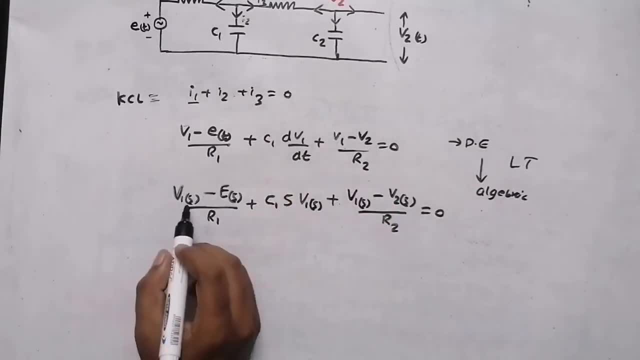 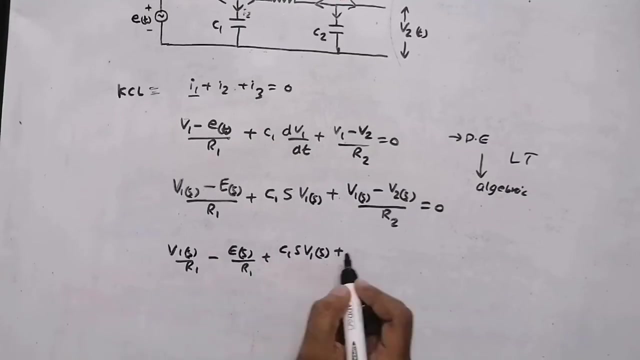 domain into laplace domain. now we can rearrange this equation. we can write the v1 or r1 times together, v1 times together. so i am going to write: v1 of s divided by r1 minus minus e of s divided by r1 plus c1 s, v1 of s plus v1 of s divided by r2 minus v2 of s divided by r2. 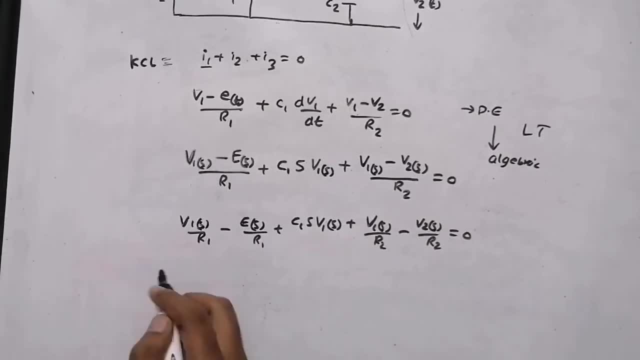 equal to 0.. now v1 is common in these three equations, so we can take v1 outside. so v1 of s i am taking outside. then here it will be 1 by r1, here it will be plus c1 s plus, here it is 1 by r2. 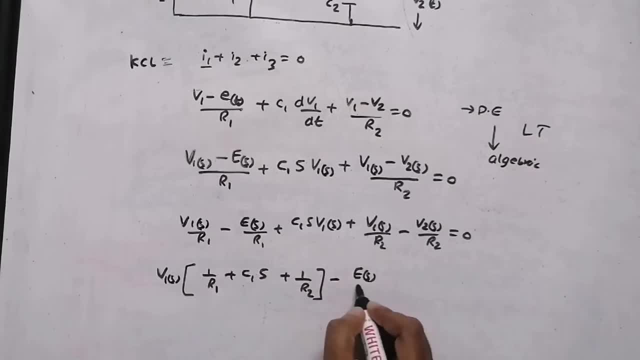 okay, now the remaining times are minus e of s divided by r1, and here it is minus v2 of s divided by r2, equal to 0. this is our first equation. if you want, we can rearrange, rearrange this equation on by cos multiplying this. so we will. 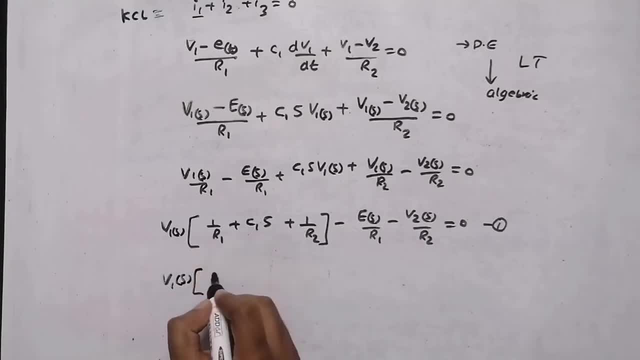 write v1 of s, then 1 by r1. cos multiplying, we will get 1 plus r. c1 of s divided by r1. okay, then the remaining time it is 1 plus r2. now, cos multiplying this, what we will get r2 into 1, it will become r2. 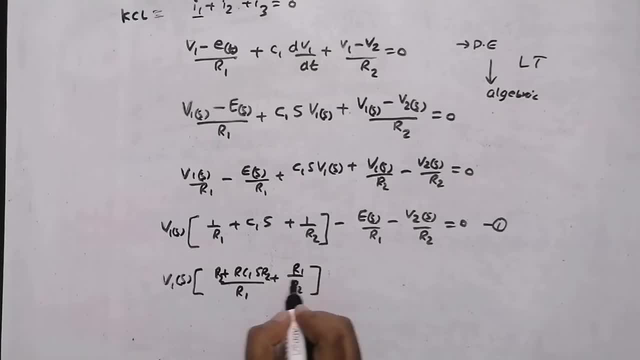 into r2 plus r1 into 1, it will become r1 all divided by r1. r2 just cos multiplied it then minus v2 by r2. i am going to write v2 of s divided by r2. now this e by r1. i am going to take that to. 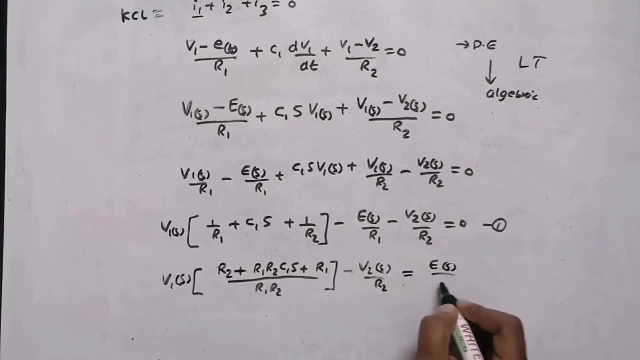 the other side. so minus will become plus, so it will become e of s divided by r1. so this is our first equation: v1 and v2, right, we wrote in this side and e we wrote in another side. so this is our first equation now applying kcl in node two. okay, node two i am going to apply, so we are going. 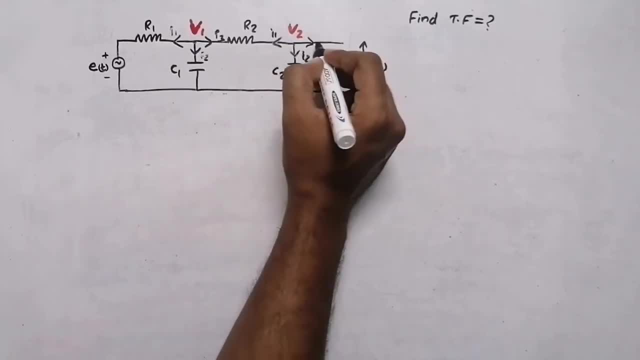 this is my current i1. this is my current i2 and i3. here it is open circuit, so current is zero. we don't want to write i3. there is only i1 and i2. i3 here it is open circuit. so first of all we can. 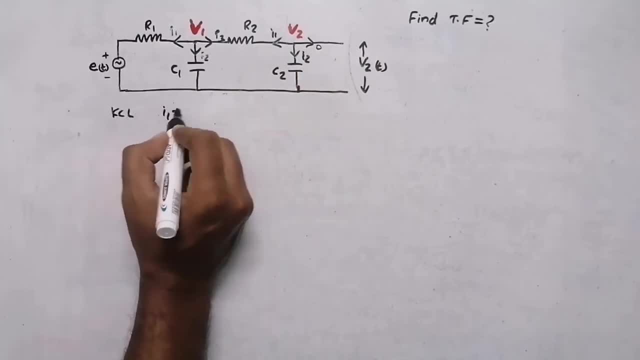 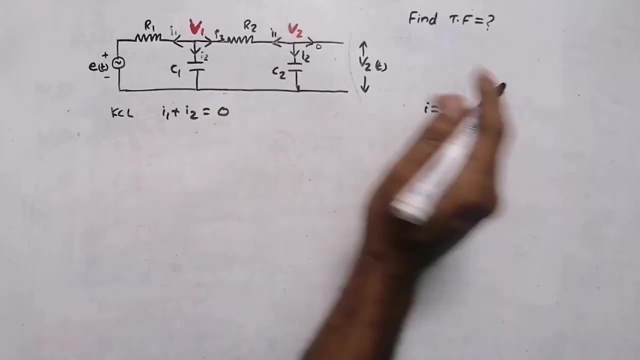 write i1. so according to kcl, what is? it is sum of current i1 plus i2 will be equal to zero. so what is i1? i1 is the current flowing through this resistor and we know current across resistor. it is v divided by r. but here there is two voltages, v2 and v1. so we will write v2 minus v1. 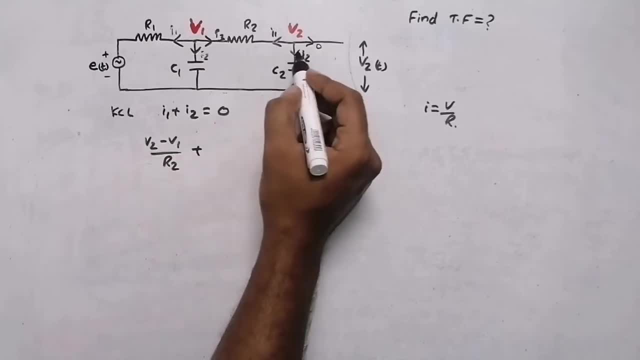 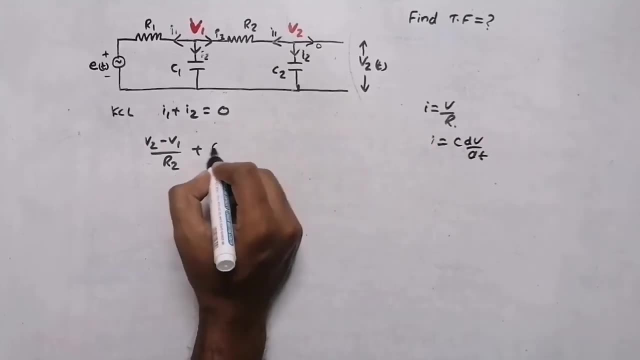 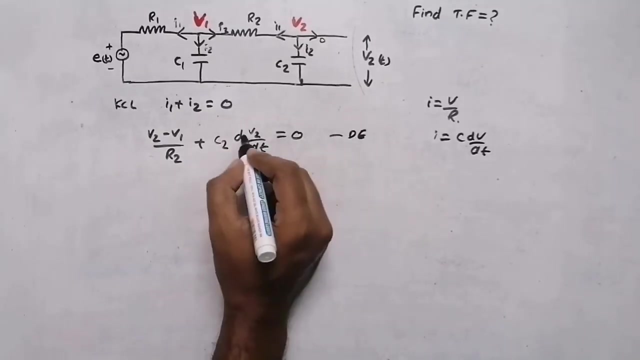 divided by r2. okay, plus i2. i2 is the current flowing through this capacitor. so current flowing is c, dv by dt. so in this case it is c2, d v2 divided by dt, which is equal to 0. now, this is a differential equation: dv by dt. okay, we need to convert it into algebraic equation using laplace. 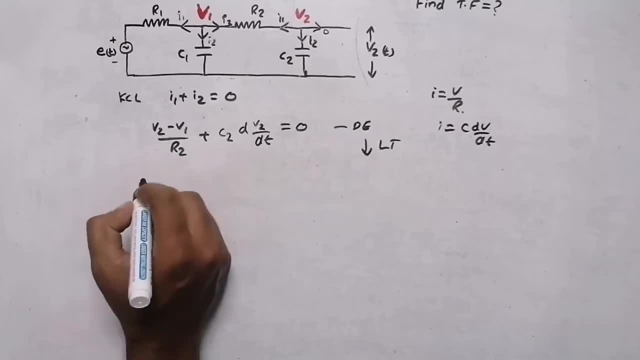 transform. so let us apply laplace transform. so small letter v2 will be converted into capital. v2 of s time domain will be converted into laplace domain. small letter v2 converted into capital v2 of s, minus small letter v1 will be converted into capital v1 of s divided by r2. r2 is a constant. 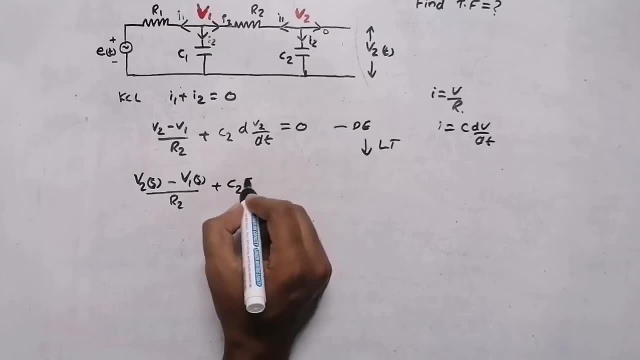 plus c2. c2 is a constant. now dv by dt will be converted into s if it is d square by dt, s square, dq by dt, sq. so here it is dv by dt, so it is converted into s and it is v2, small letter, v2. 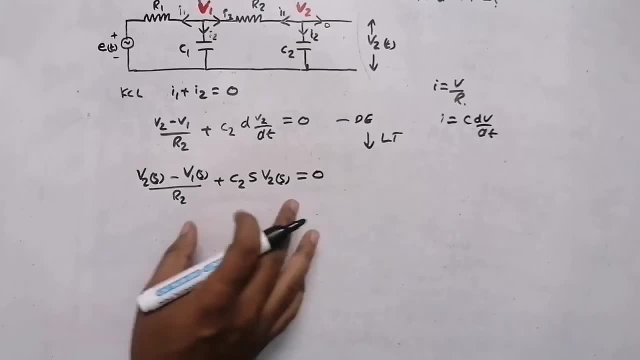 will be converted into capital. v2 of s equal to 0.. now from this equation we can split this. we can write like this: v2 of s divided by r2 minus v1 of s divided by r2 plus c2 of c2 s multiplied. 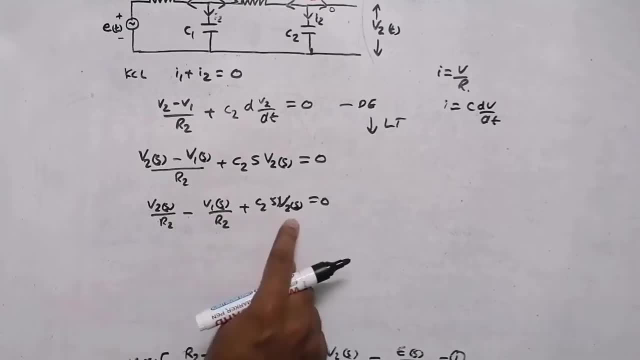 by v2 of s equal to 0.. from this, v2 is common here. okay, so i'm going to write this equation, going to take v2 outside. so i will get v2 of s 1 by r2, and here it is plus c2 s, minus v1 of s. 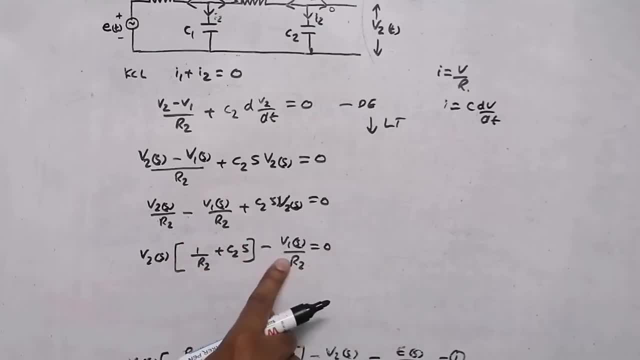 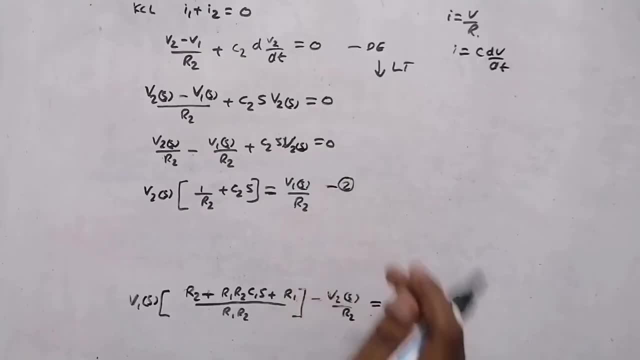 divided by r2 equal to 0.. now i'm going to take this minus v1 of s by r2 to the other side. then it will become plus v1 of s by r2. so that is my second equation. okay, now what we need to find. 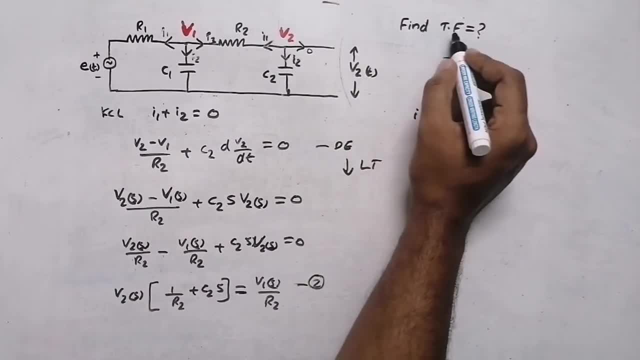 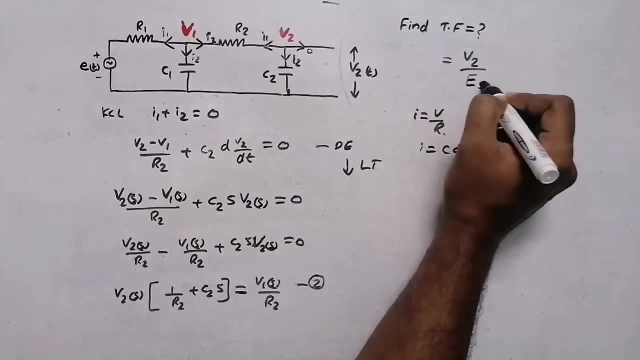 why we are writing this. we need to find transfer function. what is transfer function? our ratio of output by input. what is output? output, it is v2. what is input? input? it is e of t. so in laplace it will be e of s and here it will be v2 of s. so we need only v2 and e of s. 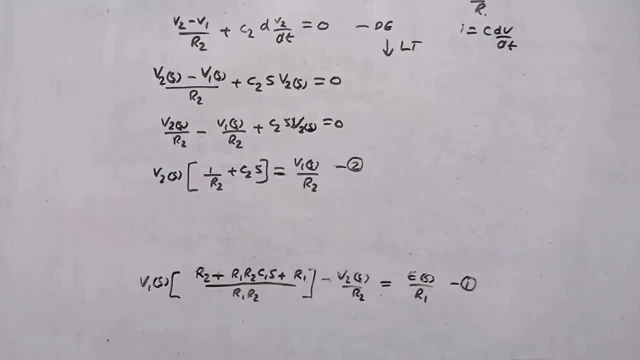 but here we have v1. in both equation we have v1. we need to remove that. how we can remove that from the second equation? we will get v1 of s. right, if you move this r2 to the side, then we will get v1 of s. i'm going to take r2 to this side. okay, now we got v1 of s. substitute this equation here. 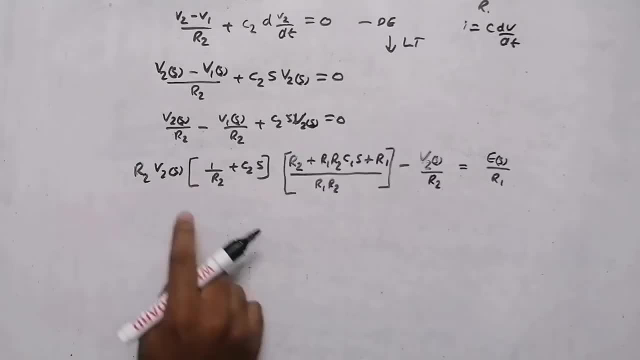 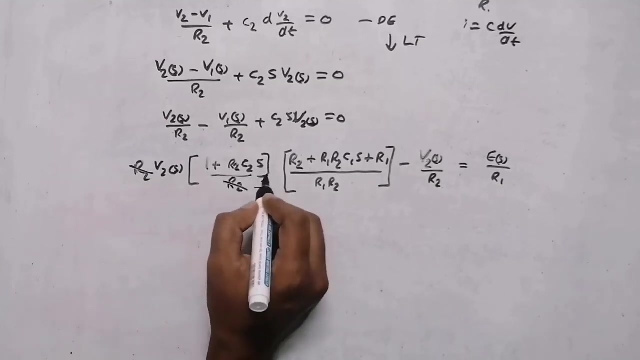 in place of v1 of s, write this equation: so instead of v1 says we substituted this. and now, in this case, multiply r2 multiplied here, then it will become all divided by r2. okay, now this r2 and this r2 will get cancelled. so we, the bracket part is over. now we can see here this v2, both. 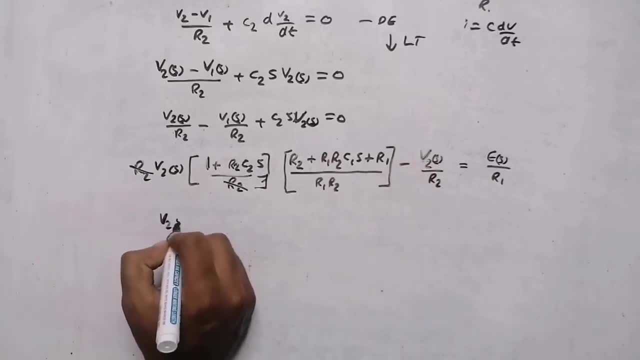 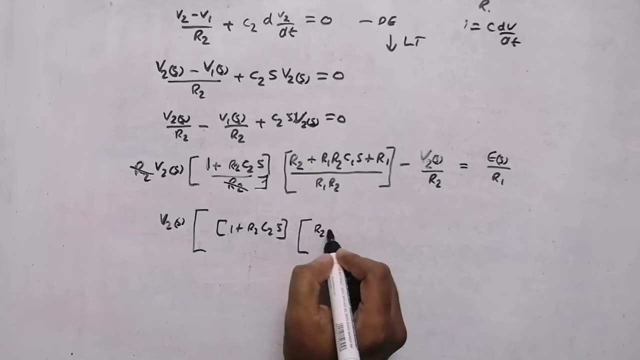 side, v2 is common, so i'm going to take this v2 outside, so it will become v2 of s, then the remaining time 1 plus r2, c2, s, then here it will be r2 plus r1, r2, c1, s plus r1, all divided by r2. 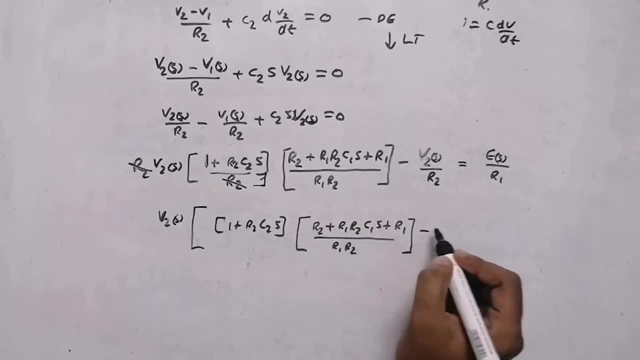 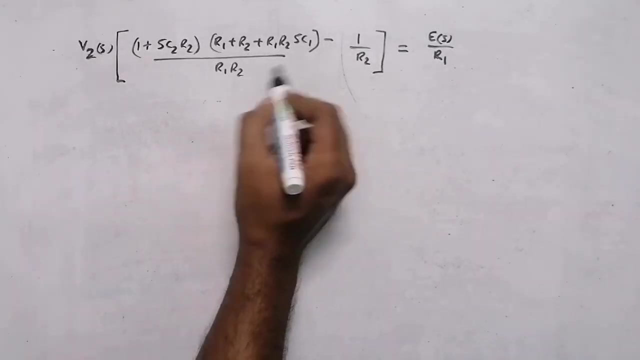 divided by r1, r2, then minus 1 by r2, equal to e of s divided by r1. now this is multiplication, so we can write: all divided by: okay, now, listen carefully. so this is the equation that we are getting. now we need to cross, multiply this. so here there is a minus sign, so we need to cross. 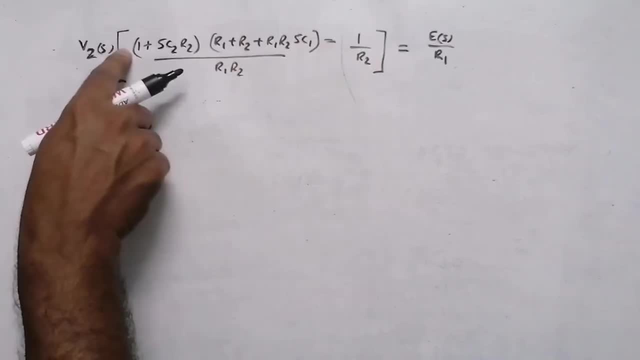 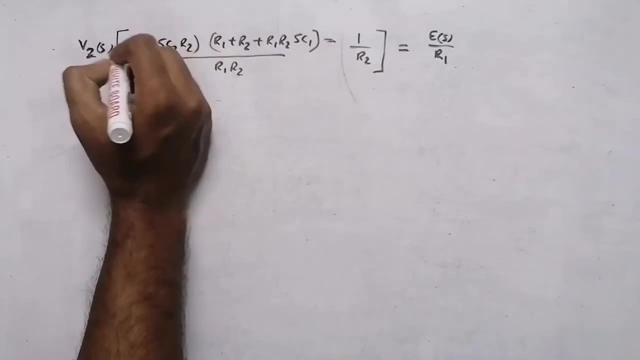 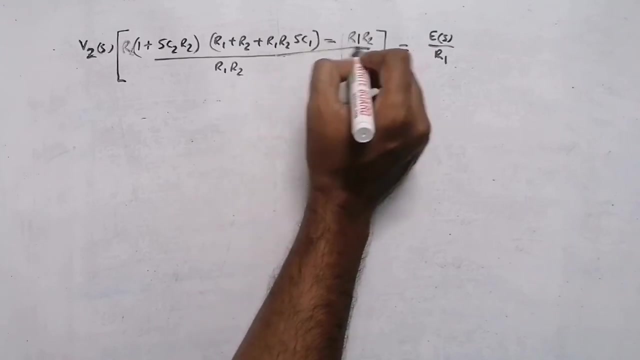 multiply so you will get r2 is r2 here and r1 r2 here. okay, cross multiply: r2 will be here, then r1 multiply here, so we can write r2 here. okay, then this r1, r2, r1, r2 here, then denominator will be all. 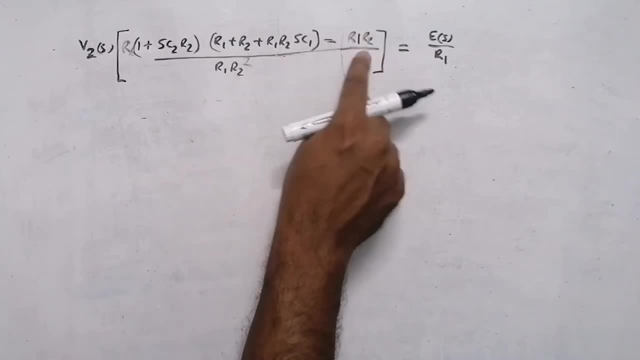 divided by now, this r2 and r2 will become r2 square, r1- r2 multiplied by r2, it will become r1- r2 square. now, as you can see, here, r2 and r2 is common, so i will take r2 outside, okay. 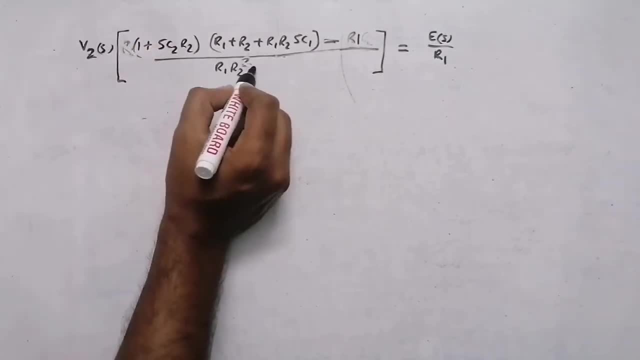 since it is common, i will take r2 outside. then this r2 and r2 square will get cancelled. okay, so r2 will get cancelled. and now listen here. here also there is r1, here also there is r1, so we can cancel this r1. the final equation: we 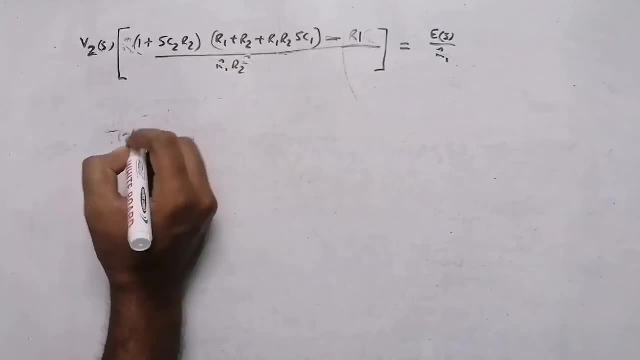 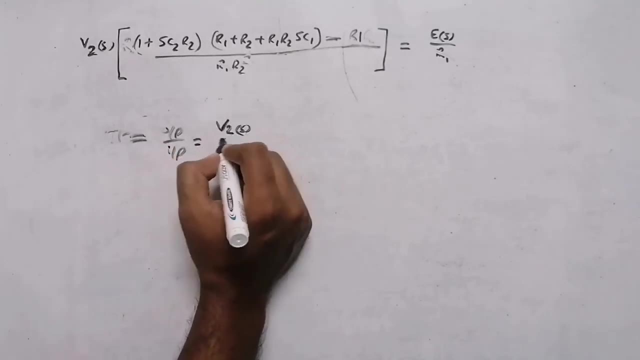 will get like this: okay, now the transfer function is ratio of output by input, ratio of output by input. what is our output? output is voltage, v2, v2 of s. input: it is e of s, so we need to write in that format. that means v2, keeping v2 here, e of s. 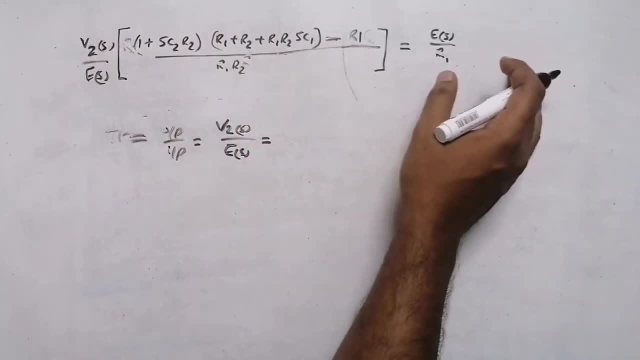 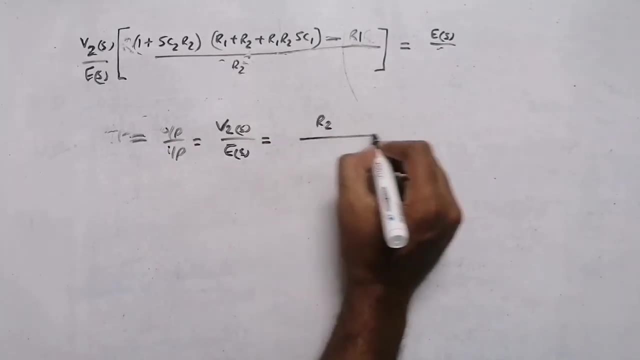 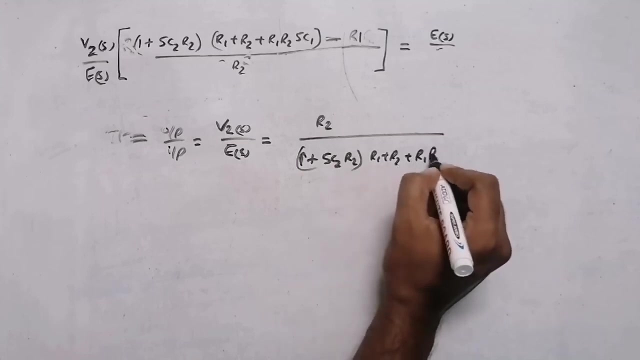 we will bring to the denominator, then this full term will move to the opposite side, or the other side. in the numerator it will be r2, because it's r1 and r1 will get cancelled. you know this: r2 divided by 1 plus sc2, r2, then r1 plus r2 plus r1, r2.